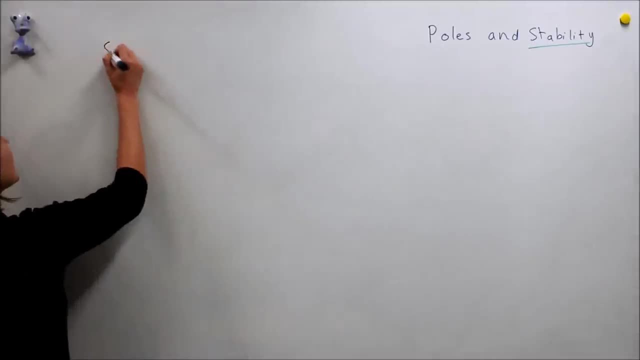 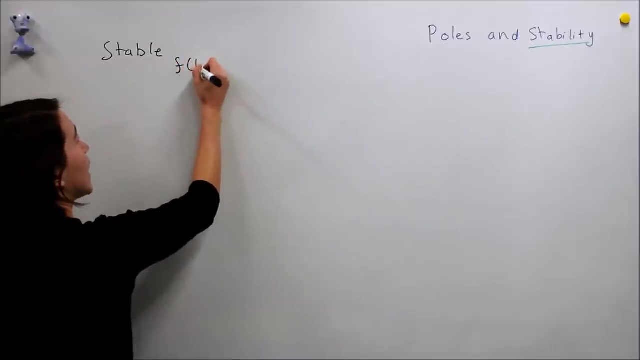 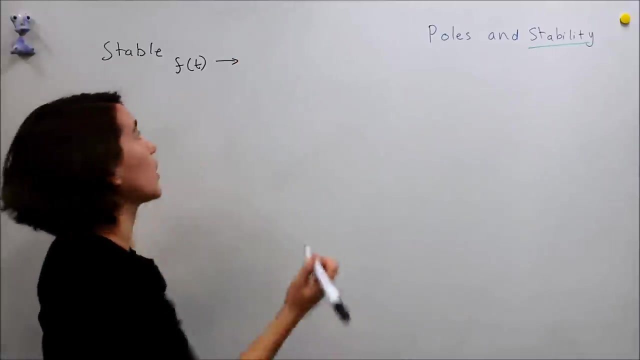 So stability is the topic, And if it's stable, it's stable. If the system is stable, say, our system is f of t. So over time we have a system And over time the system goes to zero as time goes to infinity. 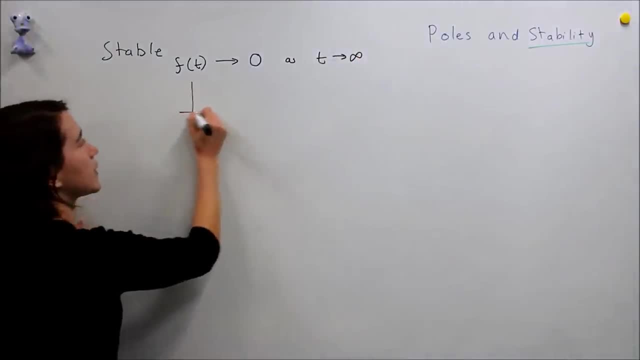 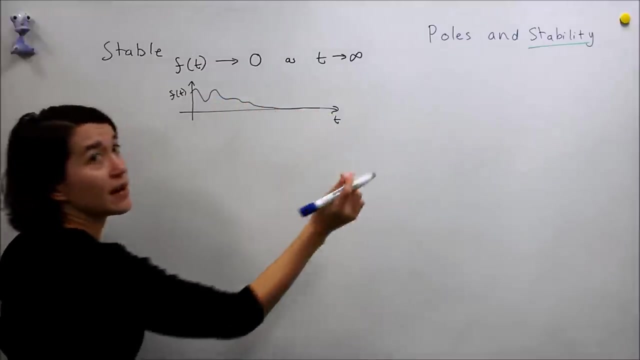 Okay, And what that looks like on a graph? we do a very generic graph here. We have f of t over time, Our system, no matter where it starts. it could start anywhere, Maybe it moves around a little bit, but eventually, as time goes to infinity, our function goes to zero. 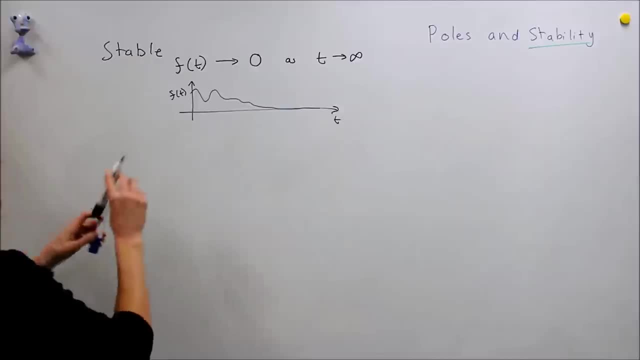 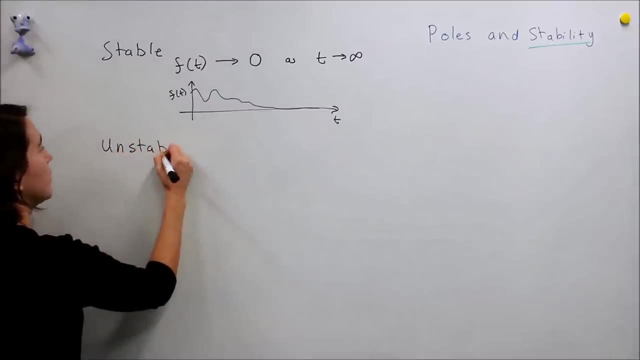 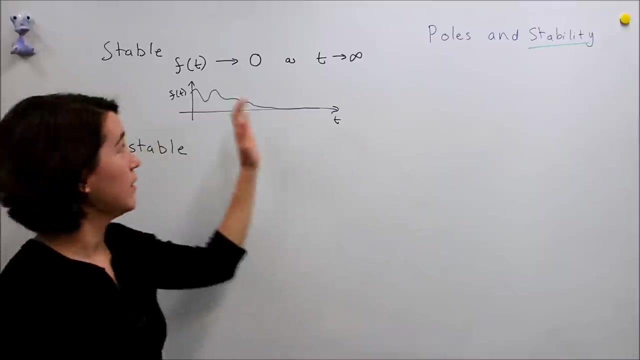 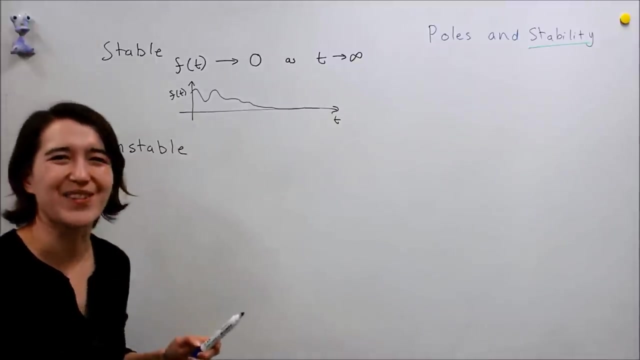 So that is stable. Our other definition is unstable, So unstable, And what that means is that our system is not going to, you know, settling down to one point, Not settling to zero. It's going off into infinity. It's essentially going to positive or negative infinity. 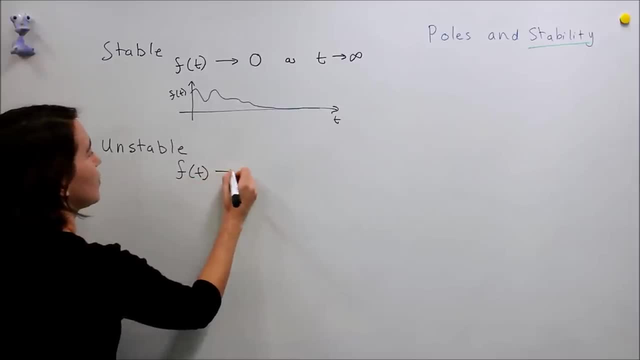 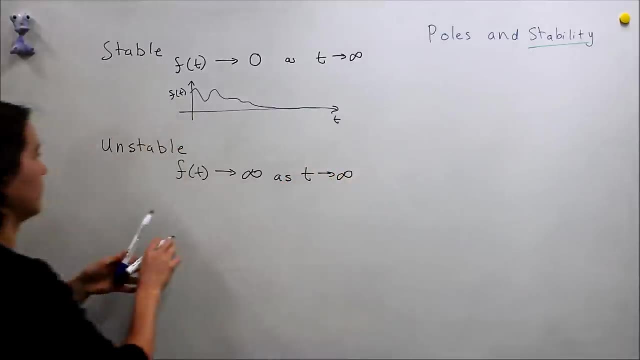 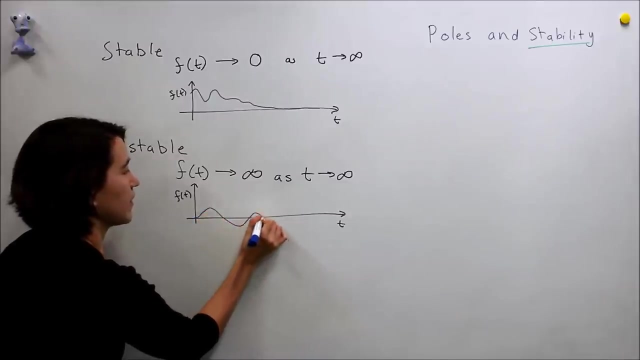 So we would say: f of t goes to infinity as time goes to infinity. So over time, f of t, you know, maybe it starts here, Maybe it actually starts really close to zero, But over time it maybe moves around but then just goes off way into infinity. 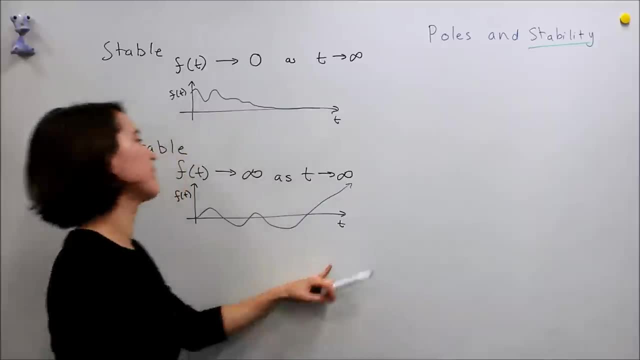 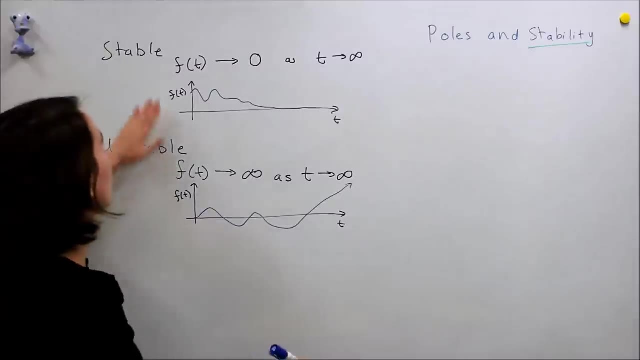 So this is what we would call an unstable system. Okay, So the next part would be: well, so we have a system. Over time it goes to infinity or it goes to zero. We've defined both of those, But what about in between? 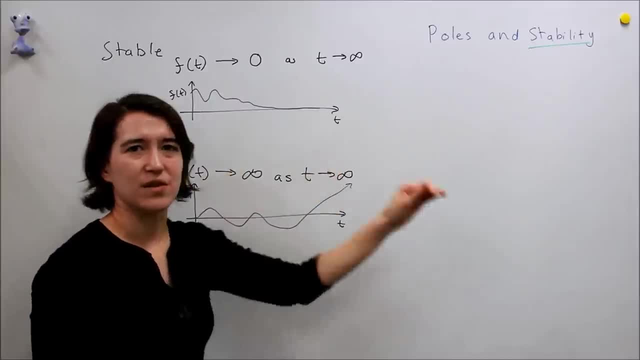 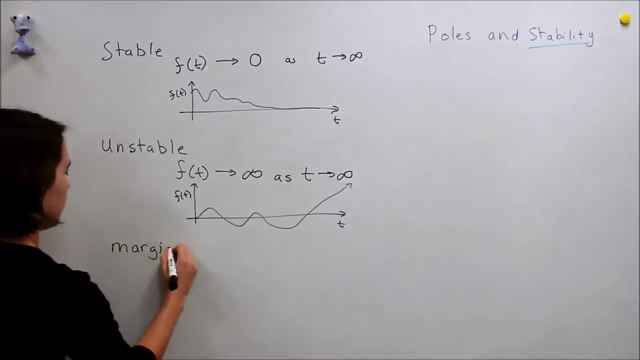 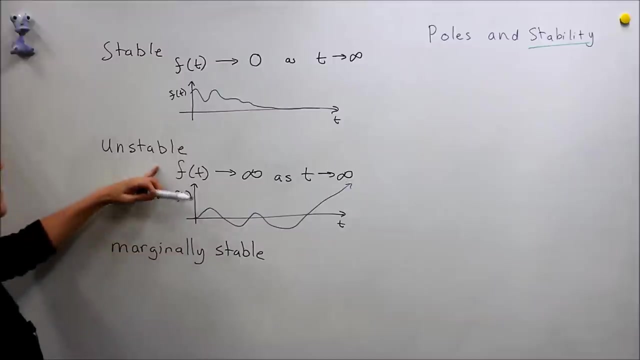 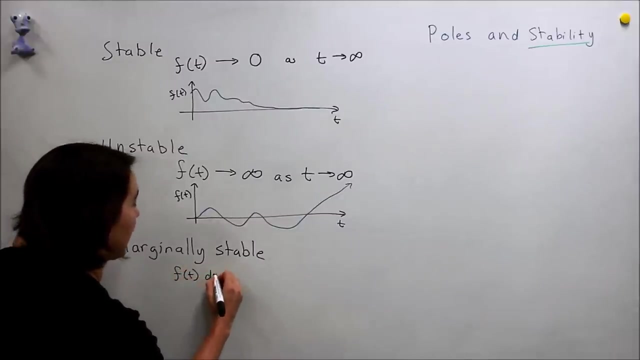 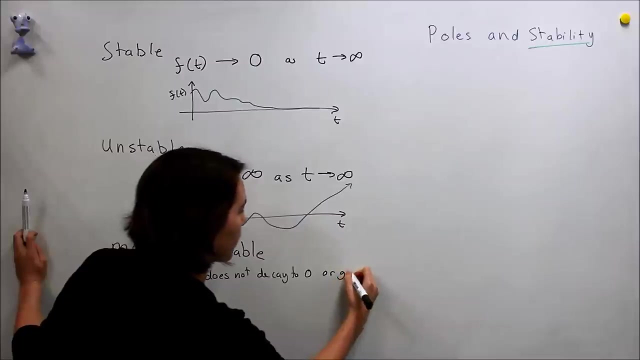 What if it doesn't go to infinity, It just goes, stays at some constant level. We would define that as marginally stable. Okay, And essentially it means it's not stable, it's not unstable by these definitions. So f of t does not decay k to zero or go to infinity. 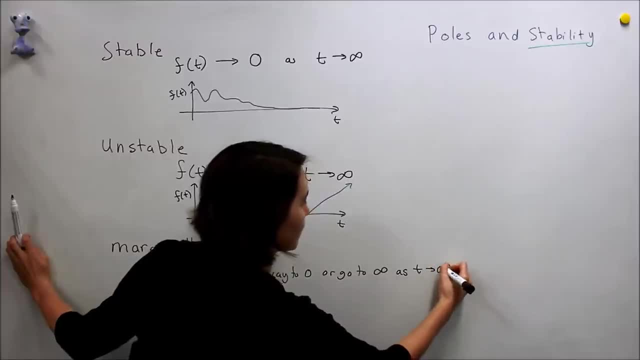 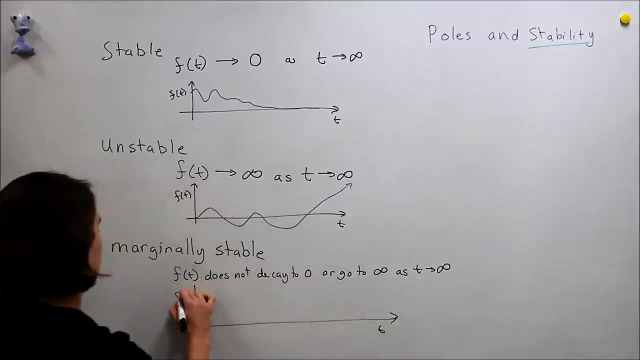 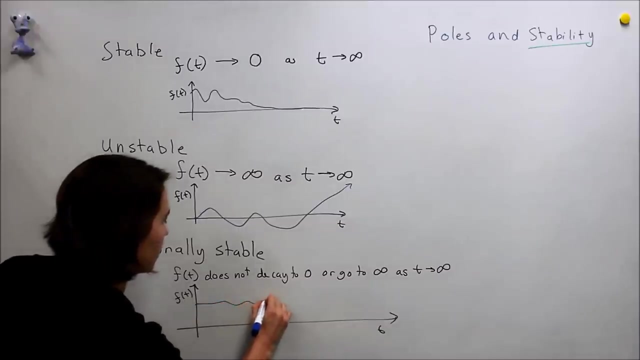 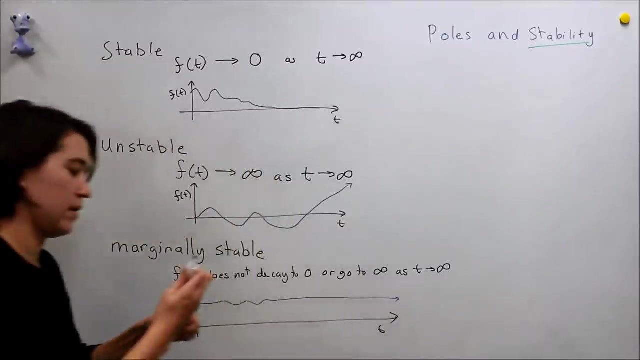 as time goes to infinity, And the two most common cases of this are that it either stays constant, So maybe it stays here and maybe it moves around a little bit, but then just ends up staying constant as time goes to infinity. The other condition which is very common is an oscillation. 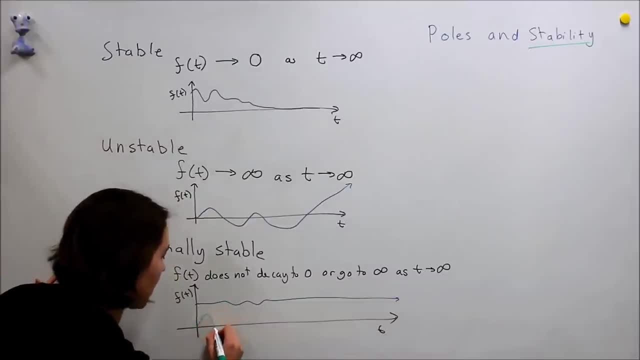 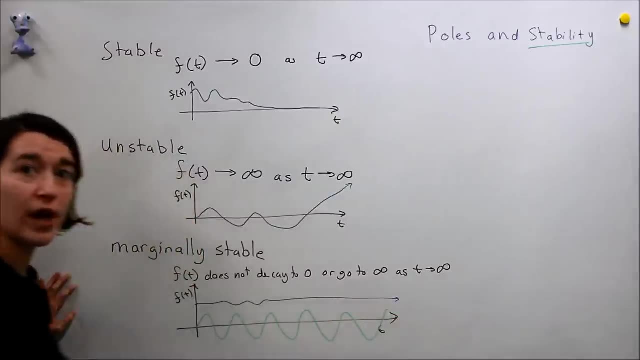 So say, you have some system and it just begins to oscillate at some resonance point and it just continues that same oscillation over time. So it doesn't go to infinity, it doesn't go to zero, but it just oscillates. 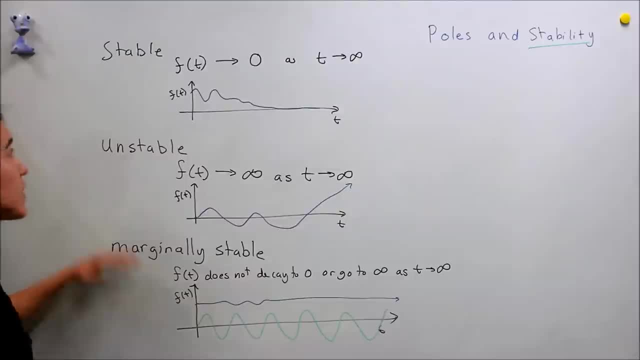 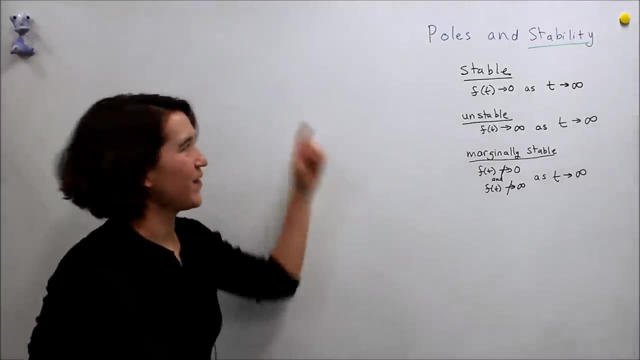 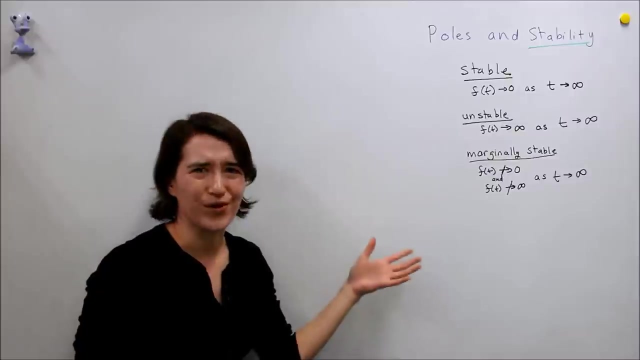 So we would call that a marginally stable system. So these are the definitions for a stable, unstable and marginally stable system. So we've defined if a system is how it's- stable, unstable or marginally stable. Now how do we relate that to the poles of a system? 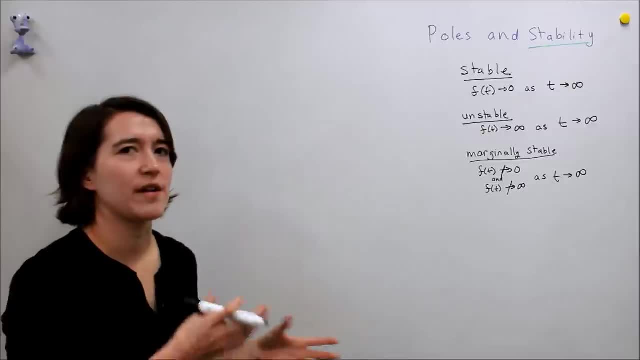 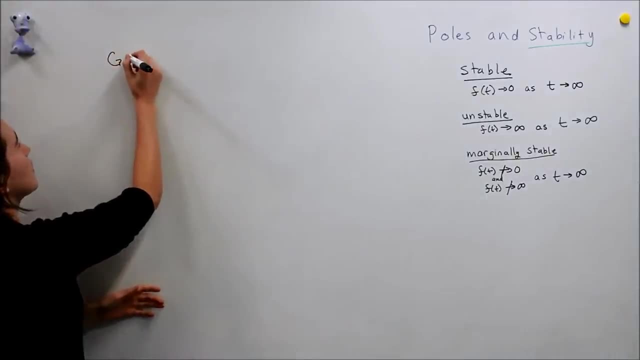 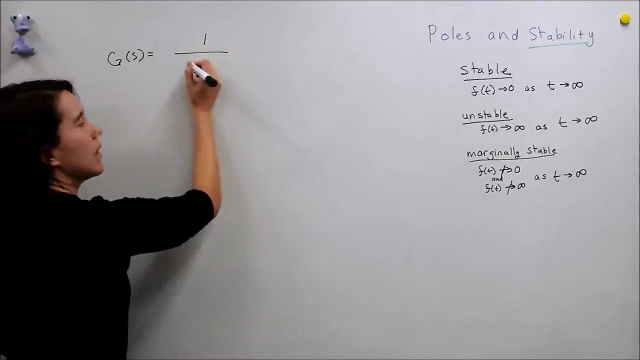 Well, we have to think back to what the transfer function actually represents. We're going to start with a really simple example. And so let's say we have a transfer function g of s and it is simply 1 over s plus some value a, some constant a. 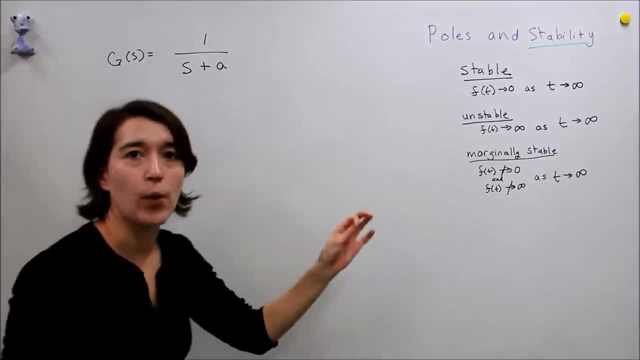 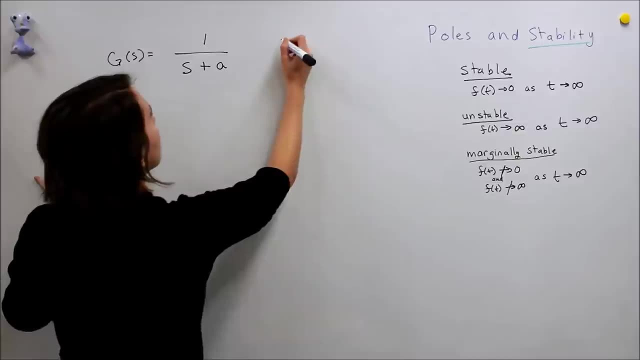 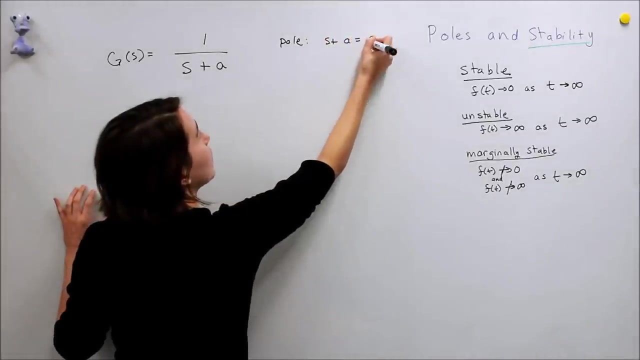 So this is a very simple system And remember from the poles and zeros we would see that we don't have any zeros, but we do have one pole. So our pole here would be whatever makes this value zero. So s plus a equals zero, which means that s equals negative. a is our pole. 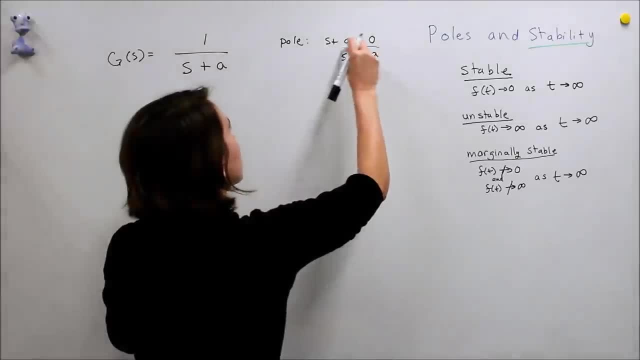 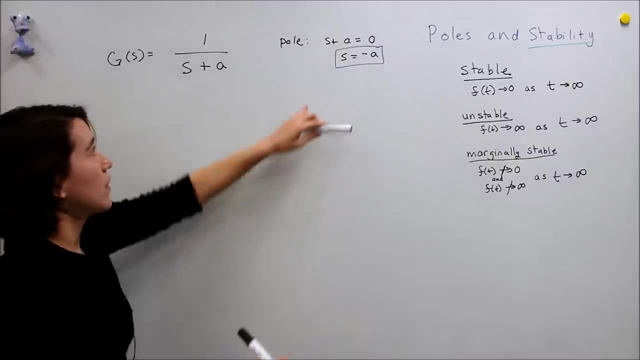 So negative a is our pole here, And we could plot that. but we need to know the value of a first. So let's think about what this means. So in the Laplace, we've taken the Laplace of this already, And so to understand what this means in the time domain, 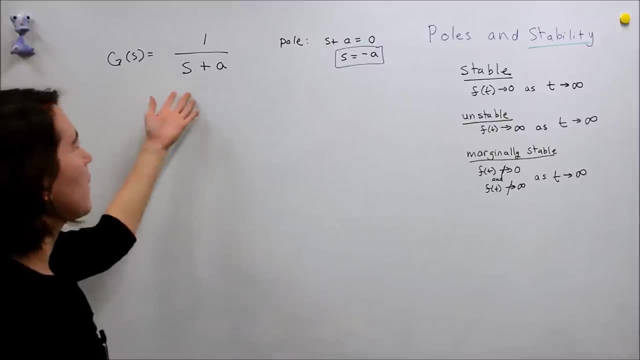 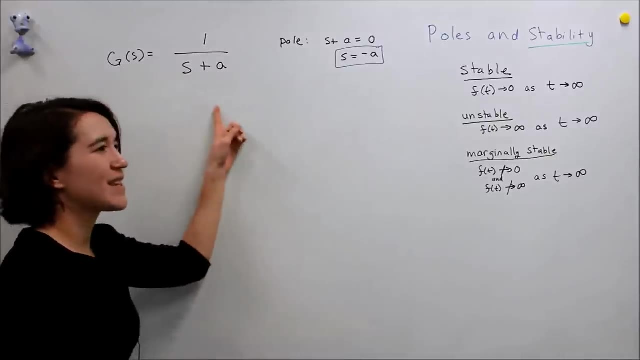 we actually take the reverse Laplace of the system. So if we remember- look at a table maybe, or if you know the systems the Laplace transforms by heart- then you can see that if we take the reverse Laplace transform of this, 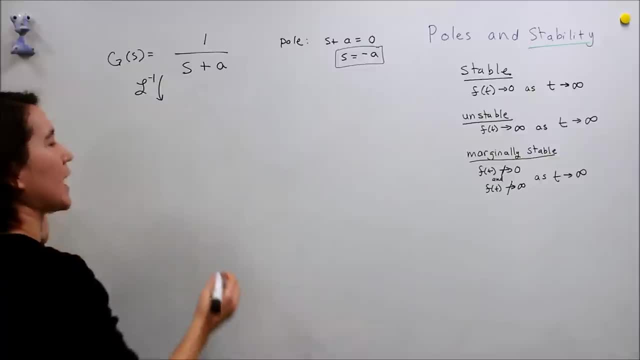 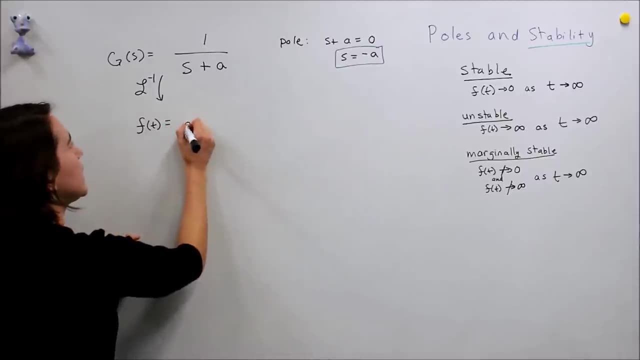 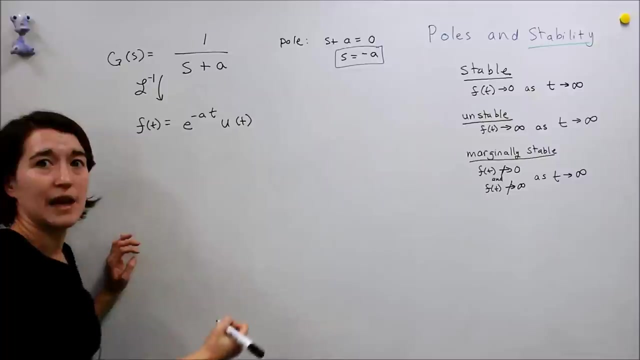 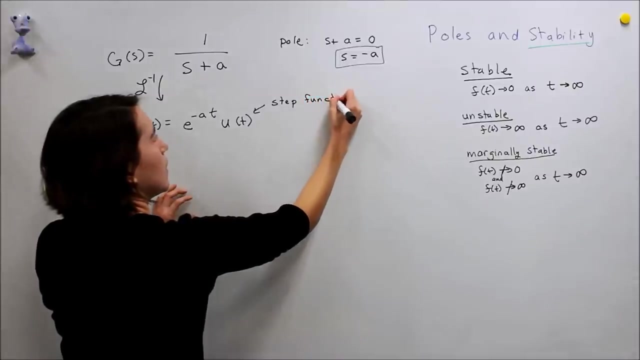 you can say the reverse Laplace we get, so we're going to call it our f of t. Then our system will be e to the negative, a t, And then we have to multiply it by u of t And if you remember, u of t is the step function. 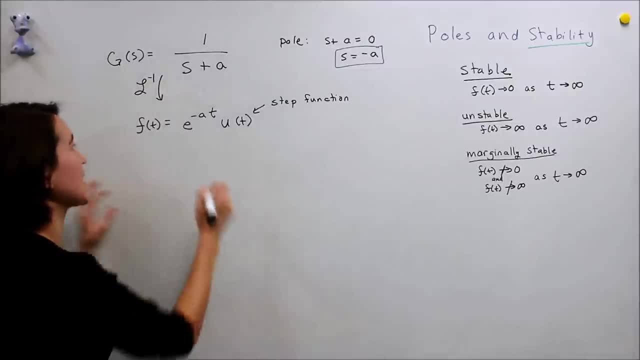 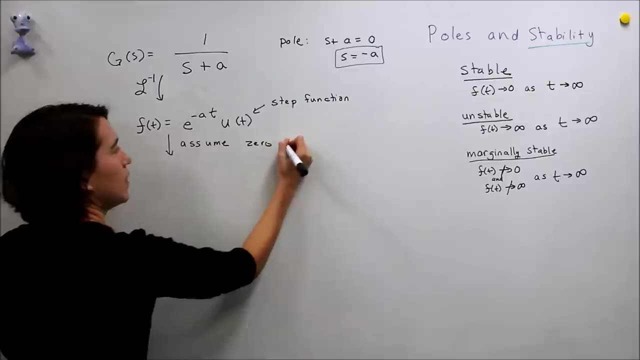 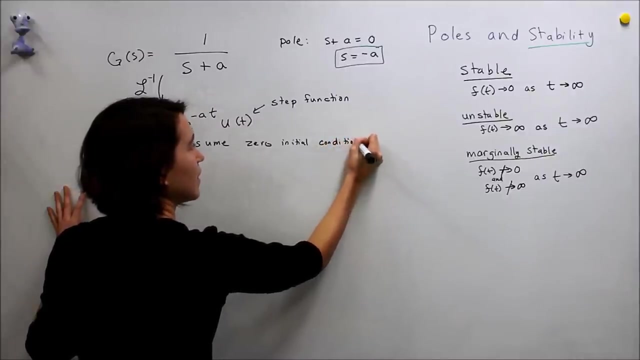 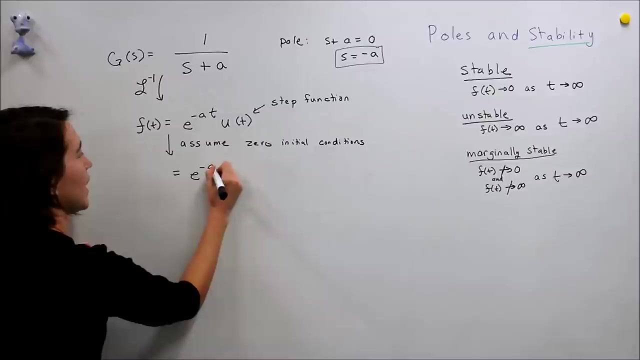 But in most systems, remember that we assume initial conditions, zero initial conditions. So if we assume zero initial conditions, then we can just make that u a, 1, and then our system becomes e to the negative, a, t. Okay, so here is our system. 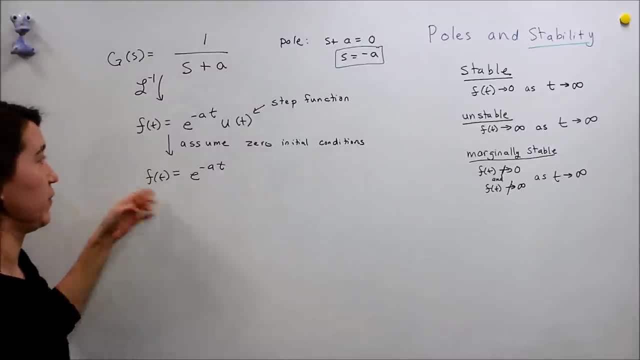 And well, what does this look like in the time domain? Well, it depends on a right If a is a positive value. so let's, let's take multiple conditions here. So let's assume that a is greater than zero. 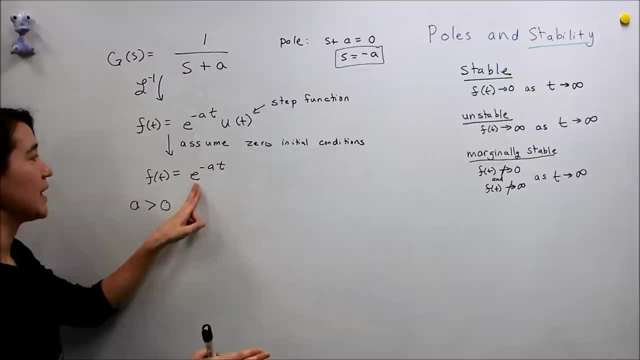 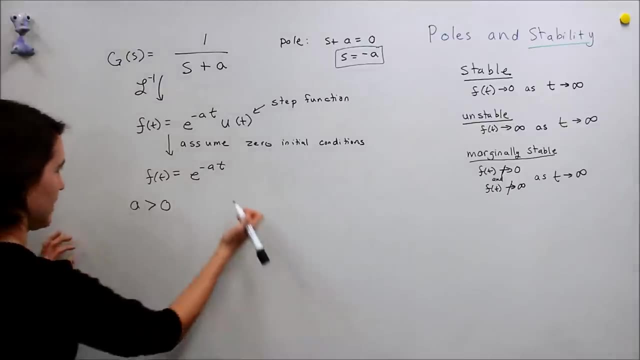 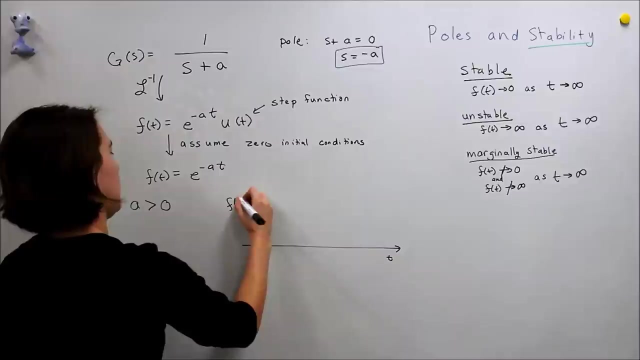 So it's a positive value. So that would mean that we have e to the negative, some negative value as time goes to infinity, So we have a decaying system. So it would look something like this: So t and f of t. 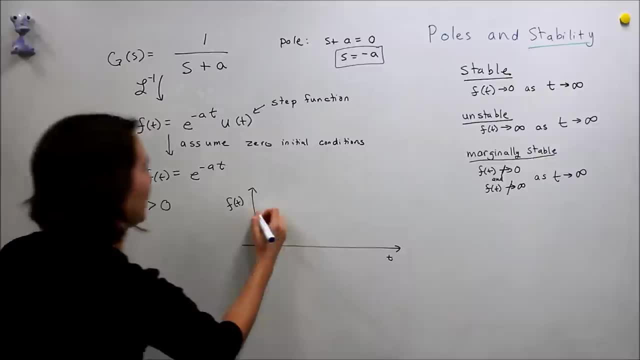 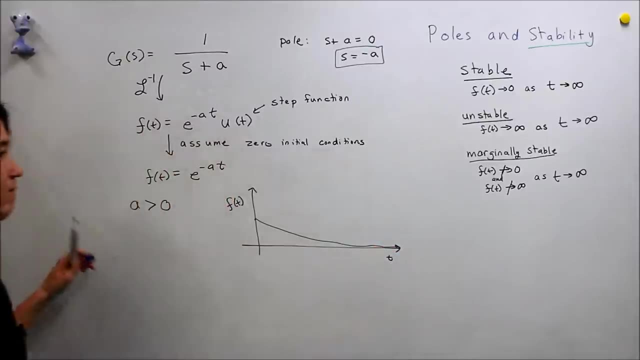 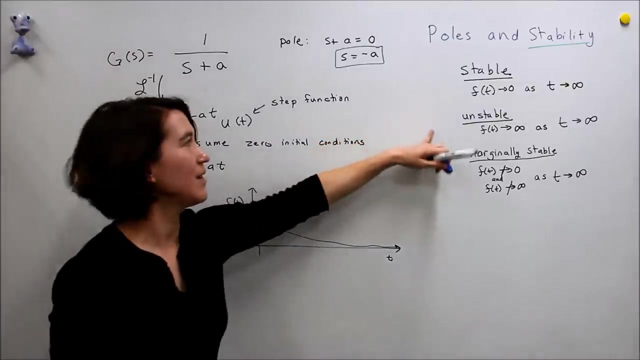 So we would have, we'd start at some point. actually, here would be one right And we would decay towards zero Right. So that would be, if we bring that back to our definition of stability, we would see that that goes towards zero. 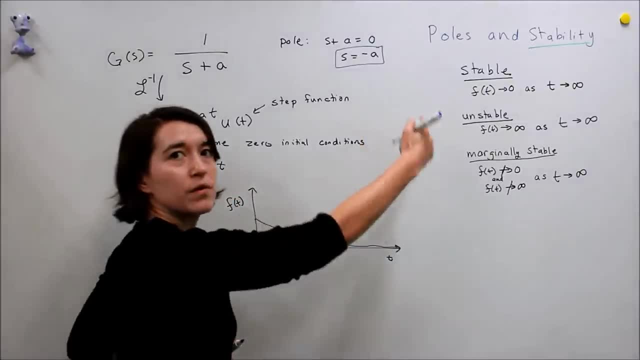 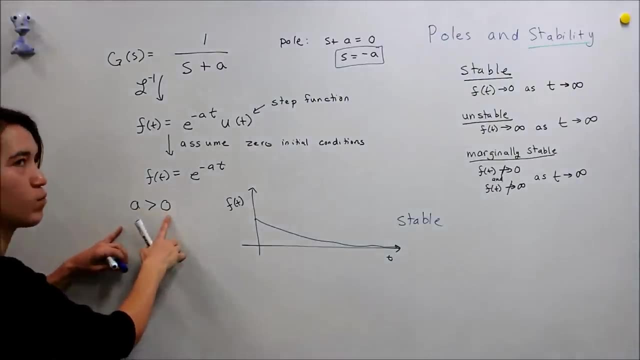 as time goes to infinity. right? This is actually a stable system. So it's stable when a is greater than zero. Okay, What about when a is? we'll do equal. a is equal to zero. Well then we have. 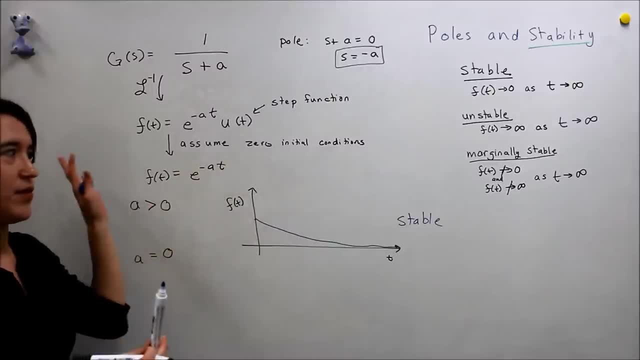 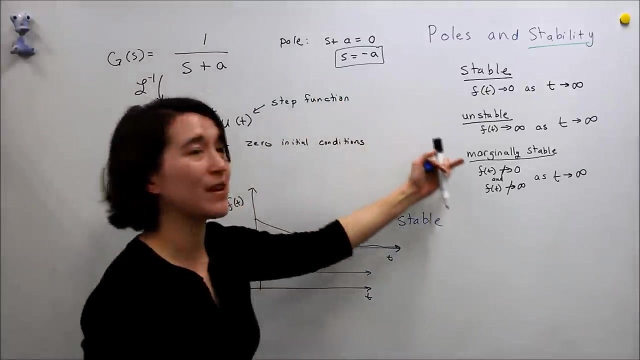 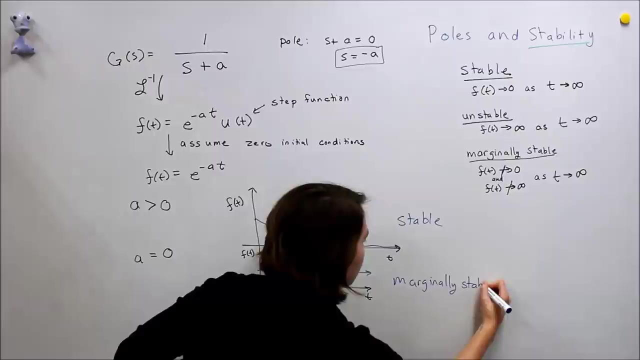 a is equal to zero. we have a one here, right? So it's just a constant one. Okay, so we would get just one to infinity, And that would be. it's not stable, it's not unstable, it's marginally stable. 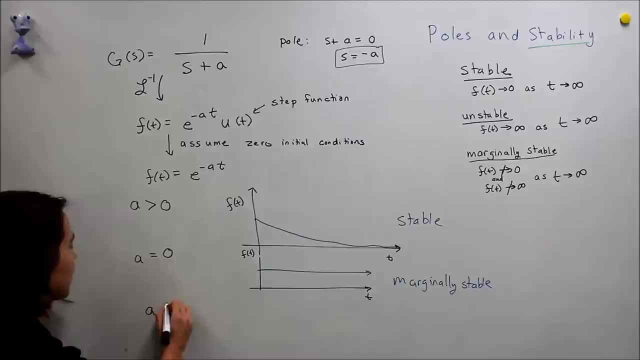 Okay. So what about last case? what if a is less than zero? So actually I should have rewritten: well, we're following this value, right? So we're putting different values of a into here. So what happens if it's less than zero? 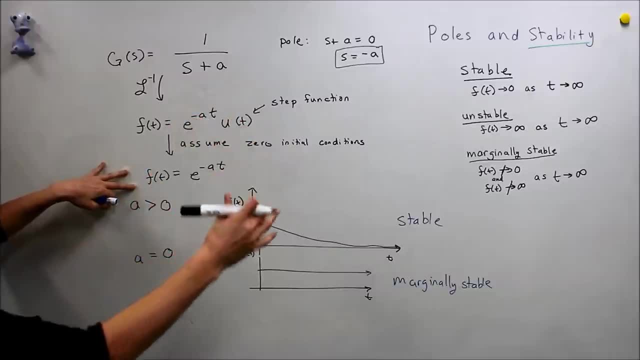 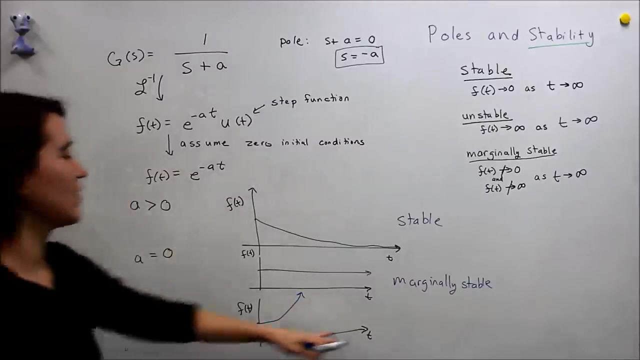 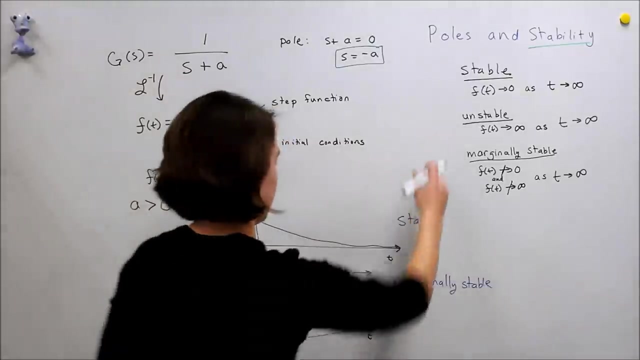 Then we have e to a positive exponential value, And that means that our function will start at one and then go off definitely into infinity. So as t goes to infinity, our value of f of x also goes to infinity. So that would be an unstable system, right? 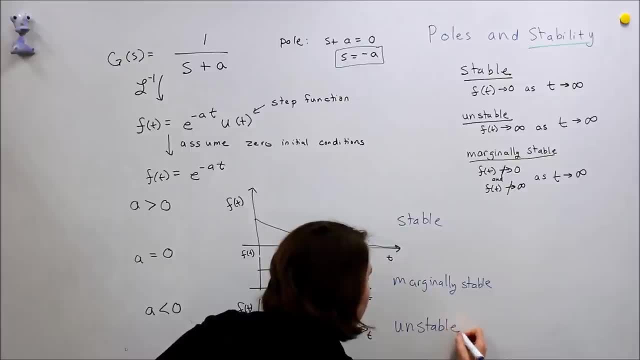 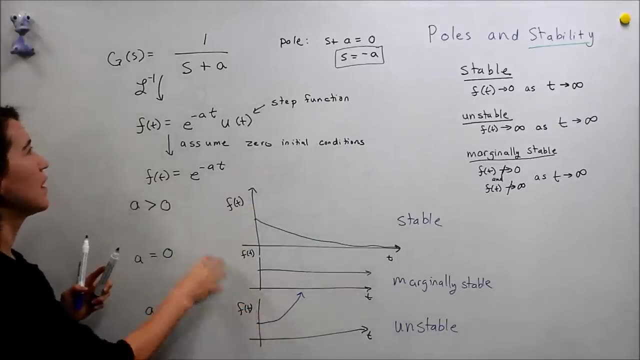 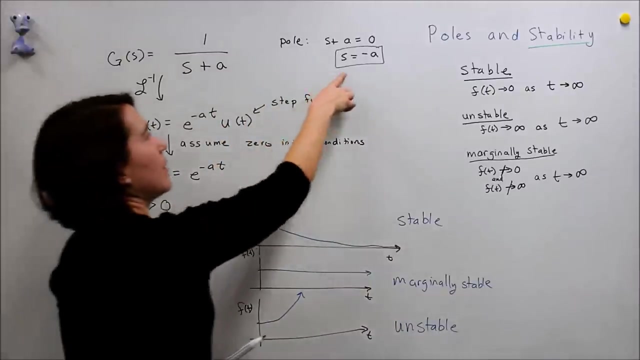 Unstable, And so we've defined these different values. We know, we understand how an exponential system reacts. If we bring this back now to our poles, we see that. so if a is greater than zero, then we actually have a negative pole. 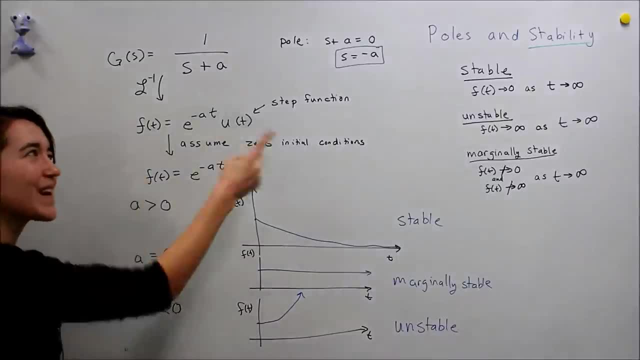 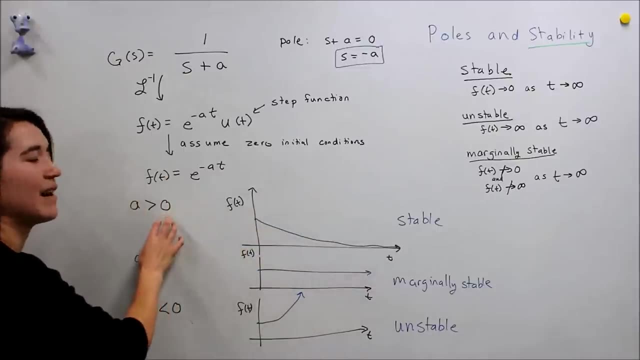 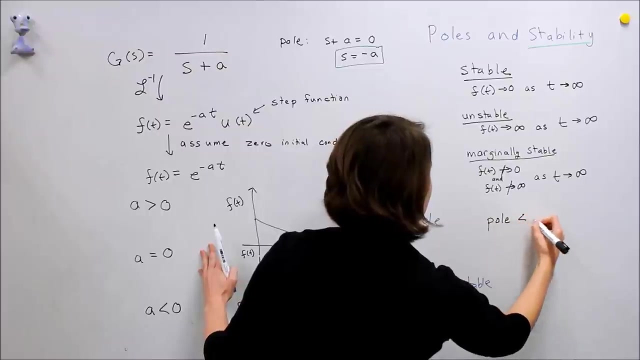 So that would be stable. So when we have a negative pole in a system, we can actually link it back through this process and see that negative pole is stable. So this is going to be a pole, a pole less than zero. Okay. 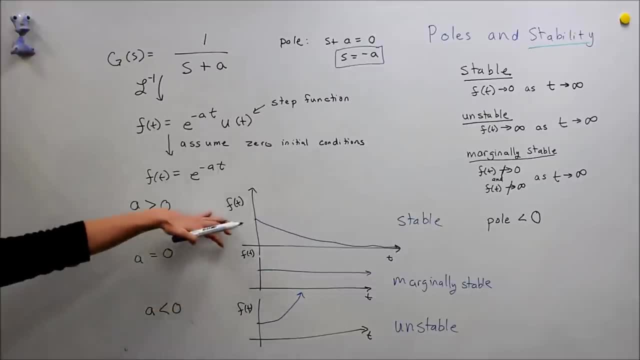 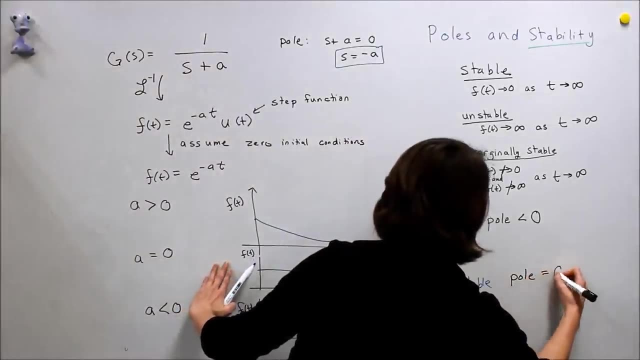 Same here. If our pole is equal to zero, we can't say it's stable, We can't say it's unstable, We can only say it's marginally stable. So this is a pole. Value is equal to zero. And here our a is negative. 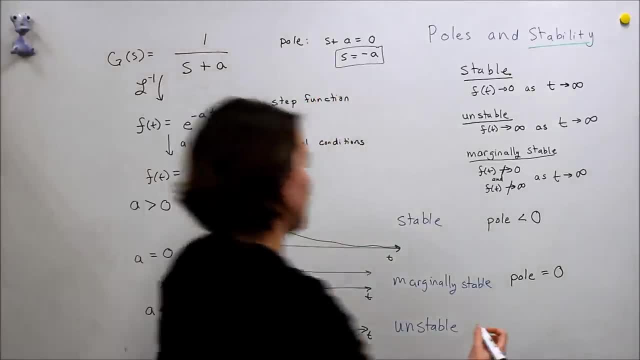 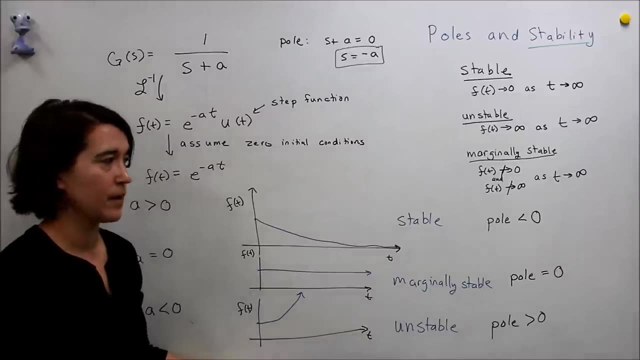 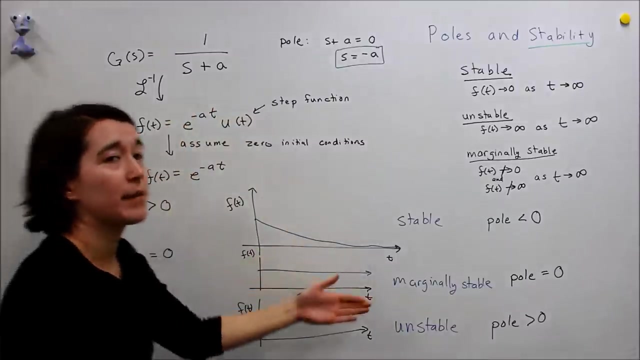 When we put it into here, it means that our pole is positive, So pole positive, so greater than zero means that a system is unstable. So from this- and we only did a simple example, but even when we applied to more complex systems, 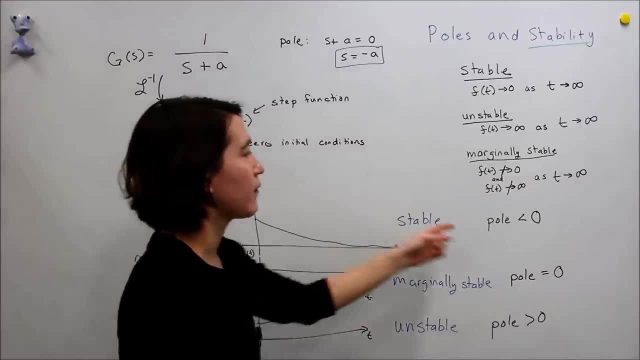 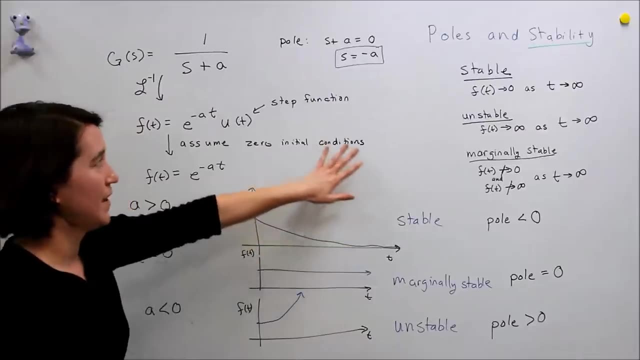 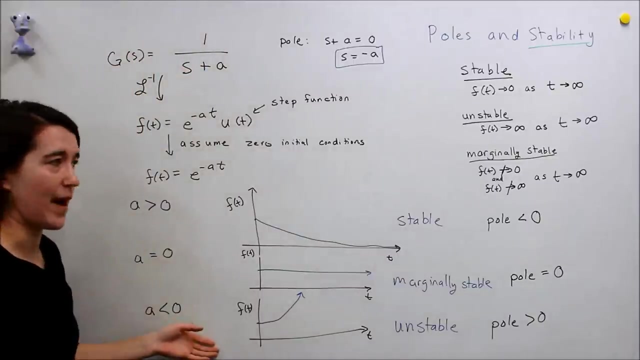 if you look at all the poles in a system and if you can find that all of them are less than zero, if they're all negative, you can say that the system is stable. So we linked the definition of stability to how the poles make the system act. 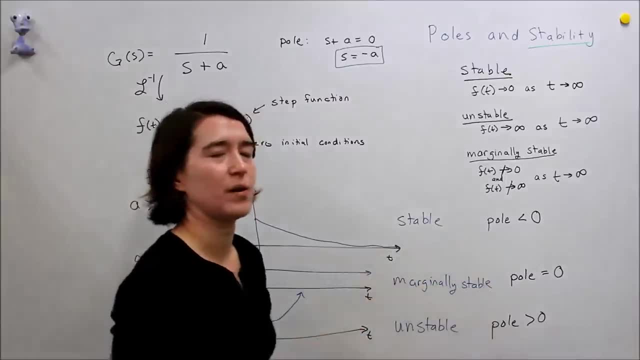 And we can look at the poles, look at their values and determine if a system is stable or unstable, or marginally stable.